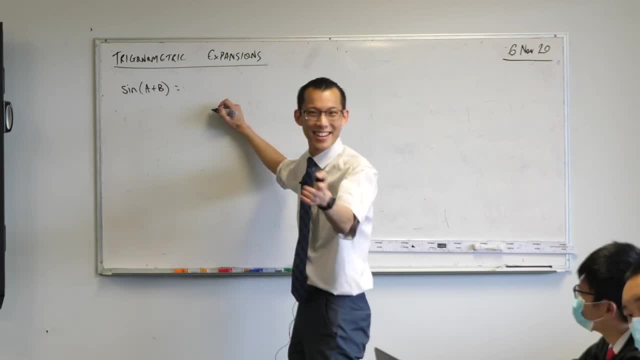 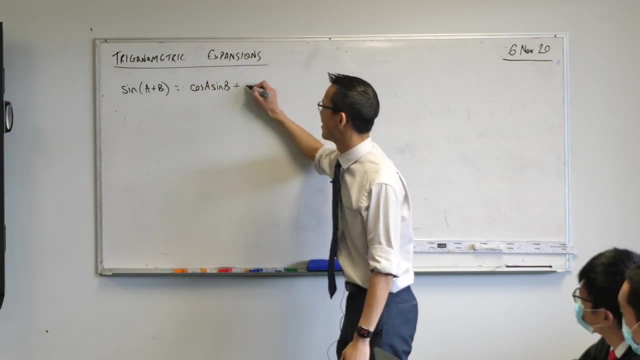 Yeah, go ahead, Ariana, yeah, Oh, shoot, Yeah, yeah. yeah, Calvin, do you want to help her out? Cos a plus, I mean cos a sine b plus sine a cos b, Very good, Okay. so if you haven't got that down, you should write it. 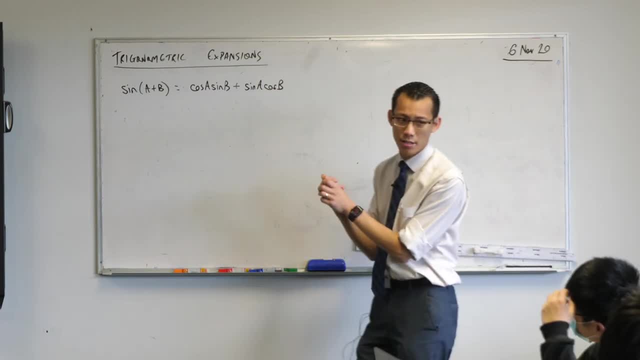 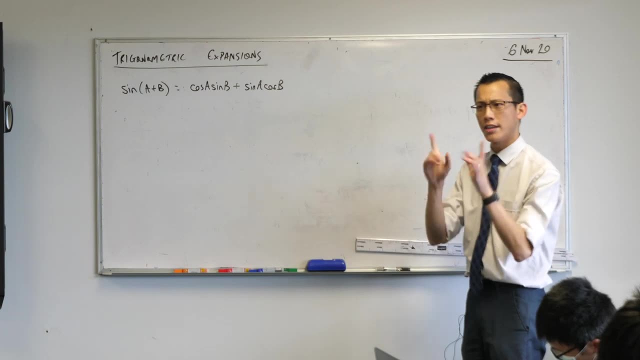 This particular result, by the way, on the reference sheet. but you'll use this enough. at least, I hope that you won't need to refer to that anymore, though it's nice having a security blanket, Now I'm going to ask for a show of hands here. I will not put you on the spot and ask you to actually do it. 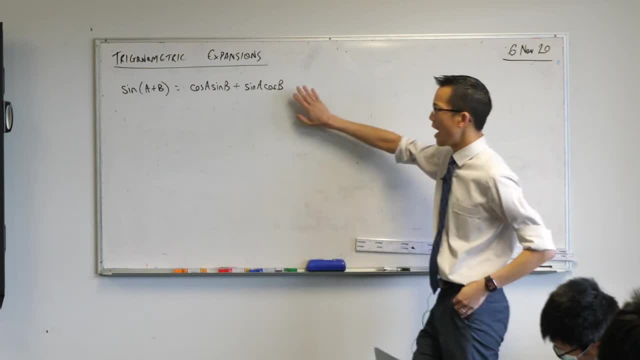 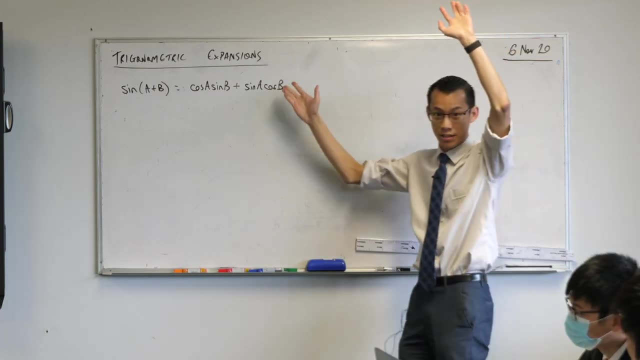 but I'm just curious to know how many of you have an idea of this, How many of you could say to me I know why this is true. I could explain it to someone else and prove Not that it is true and accept it, but I can show you why. 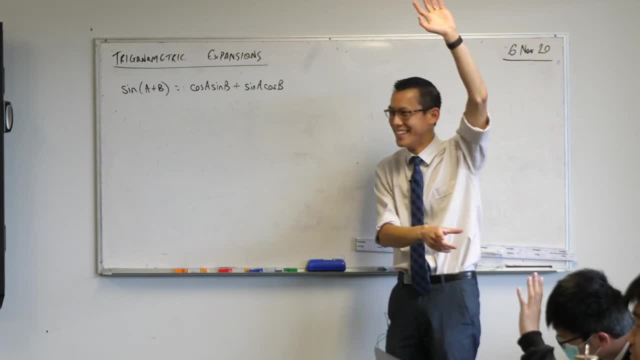 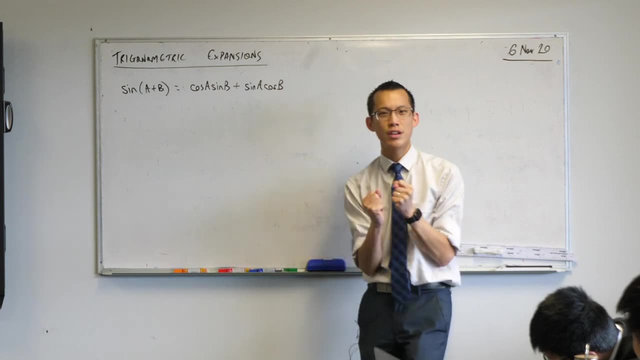 Anyone, Any takers? I see one, Two, one and a half. Anyone else? Okay, interesting, Thank you, Hands down. What I want to say to you, firstly, is that should unsettle you just a teeny little bit. 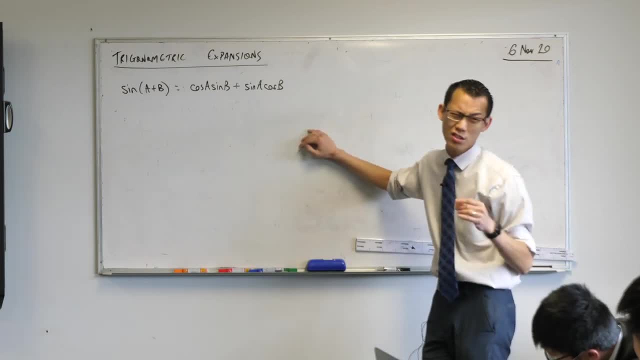 Throughout mathematics, especially when you look at something like that, there are some bits where, especially when you first learn it, you just accept it. You're like, okay, you know, Mr and Mrs Lees, they've never lied to me before. 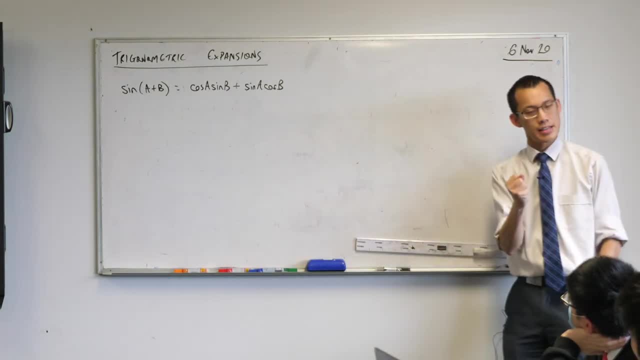 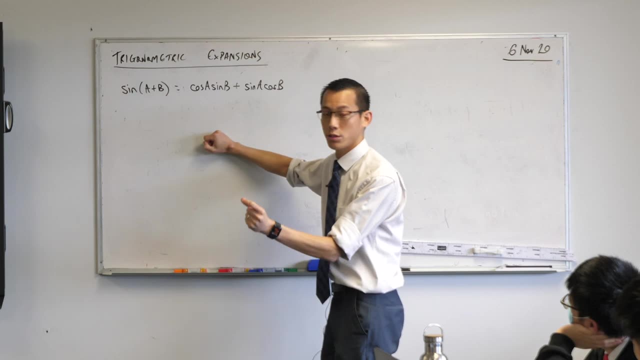 I'm just going to take this as given right, But one of the things- it's actually one of the design principles underneath this entire course- is that every result you ever get handed, you know enough mathematics to prove it for yourself and not just trust someone else- a textbook, a teacher, whatever. that it must be true. 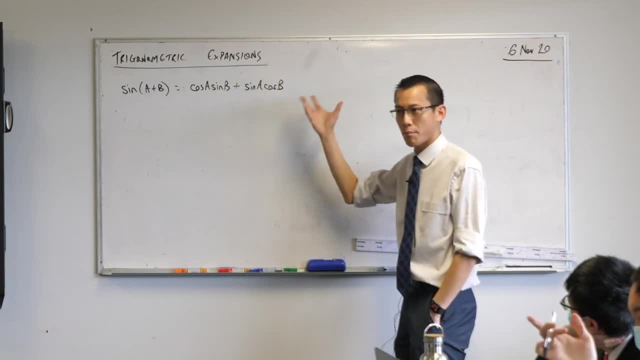 Now you actually have, I hope, been shown some form of a proof, some derivation. It probably had some weird triangles, maybe the unit circle in it. It's a bit of a complicated mess is what I'm trying to get at. 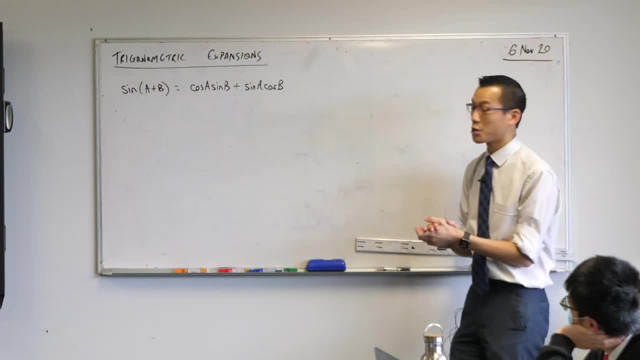 It's why so few of you actually can say: oh yeah, I know right. So what we're going to do is we're going to prove this result, and all the rest of them as well, remarkably quickly using complex numbers. 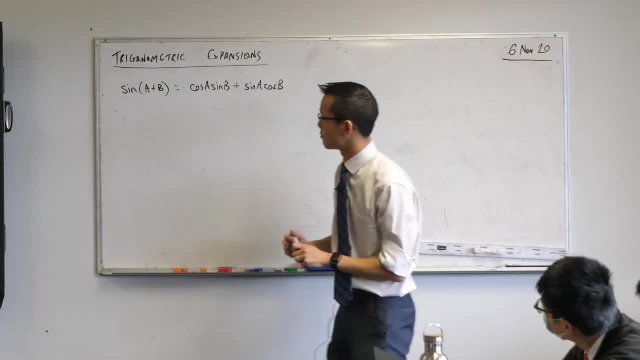 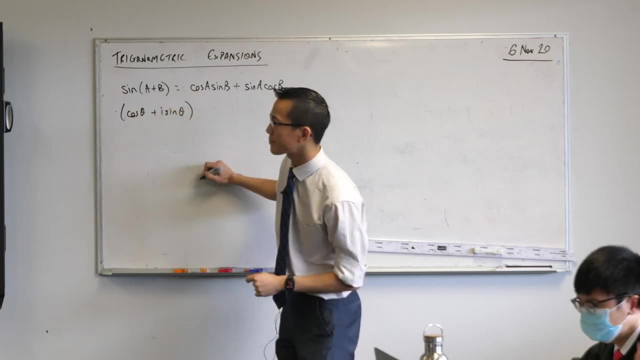 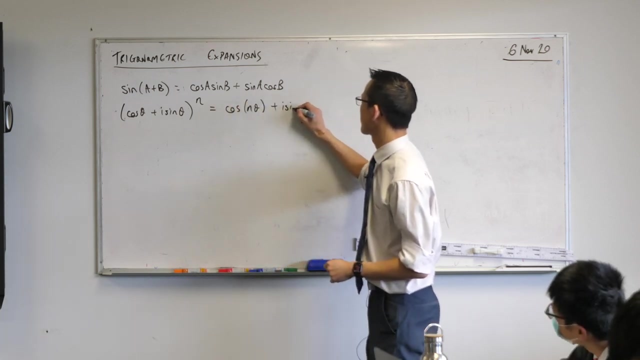 So what I'm going to do is take you back to DeMarvin's theorem, right? So we've got this guy here. cos theta plus i sine theta to the power of n equals this guy here. We're going to use this as an example of how to get to. it won't be this one first. 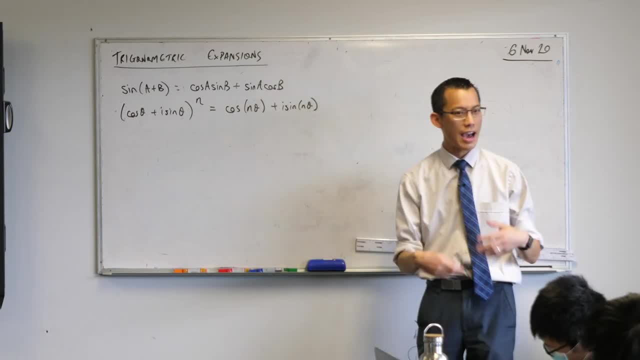 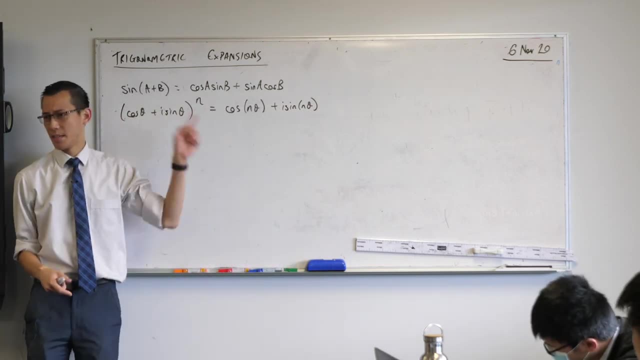 but it's going to be an example of this that you'll see how quickly it comes out of our use of complex numbers, right? So simple example, right? This guy here. it's a bit of a mess, so I want to try and come up with a simpler version of it, right? 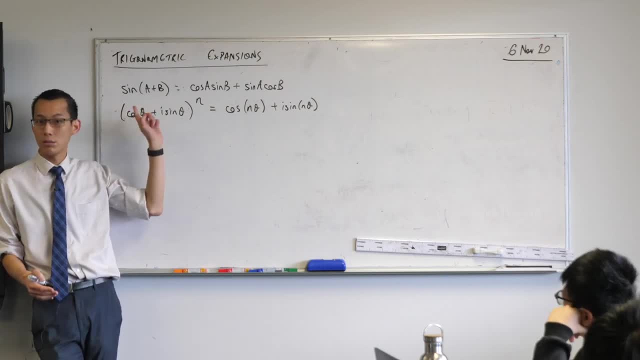 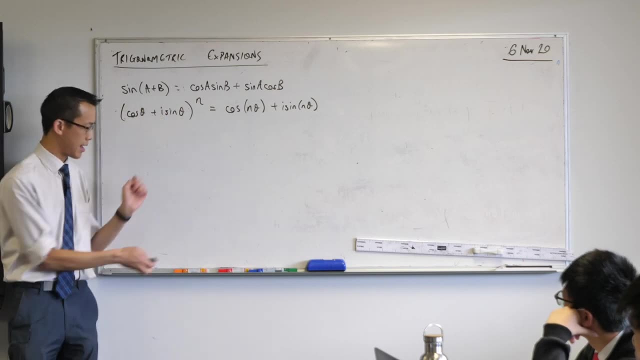 So I wonder if you can imagine with me what would happen if both of the angles, the a and the b, what if they were the same angle? Like what if they were the same size? okay, So this is a particular version of sine a plus b. 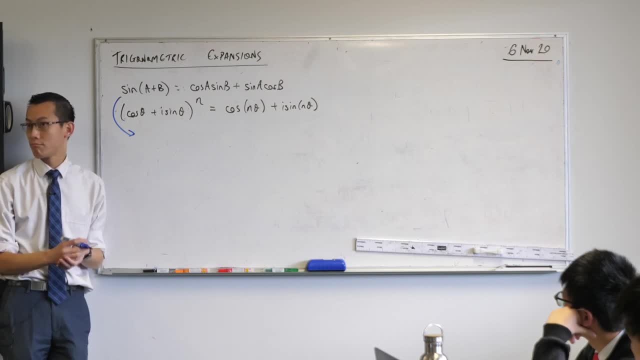 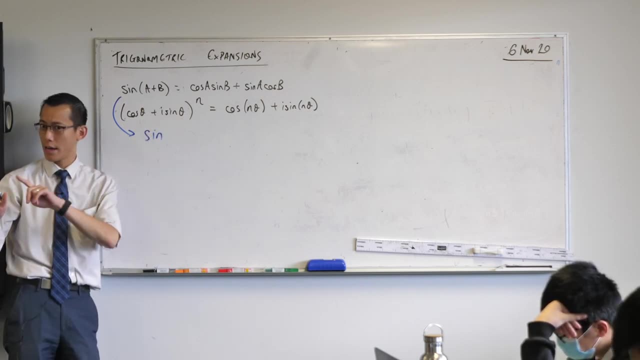 where, if we call both angles, say equal to I don't know alpha, okay, If I made them the same, then you'd have alpha plus alpha, so that'd be sine two alpha, do you agree? Now? hopefully you can interpret this line well enough to say: 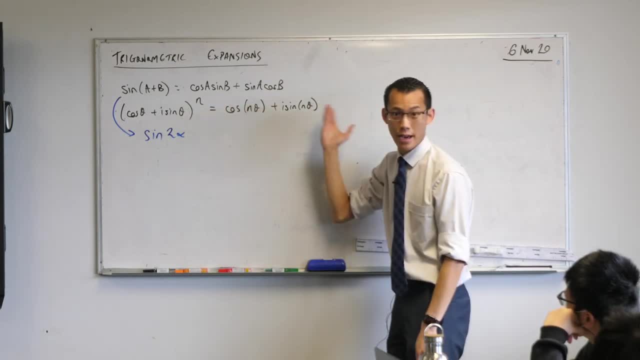 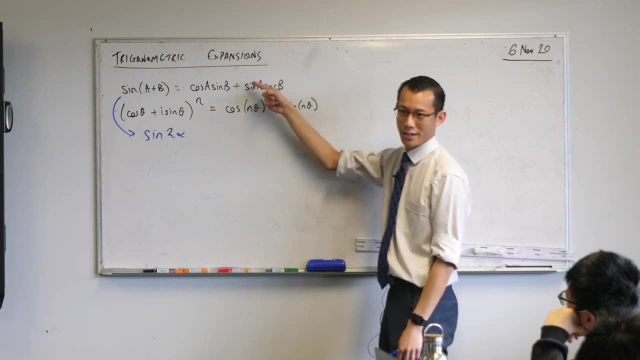 if I just substitute alpha into everywhere I say a and b, you'll get a result out. okay, So this is what we call a double angle trigonometric expansion or double angle formula. Now what I want to get to like. I know you can already do that just by putting it in there. okay, 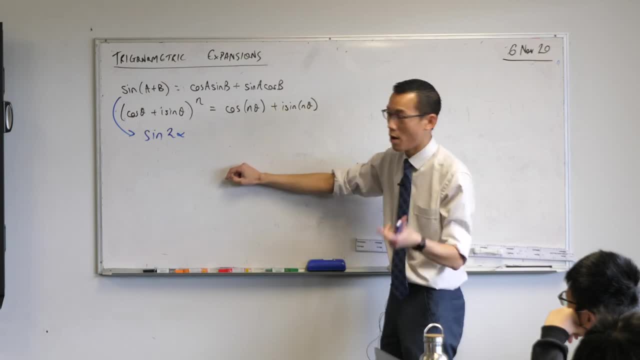 But you don't know why this is true. so I want to try and get at why, and we're going to use this to get there. Okay, how will I use this line- Demarva's theorem- to try and get a result? 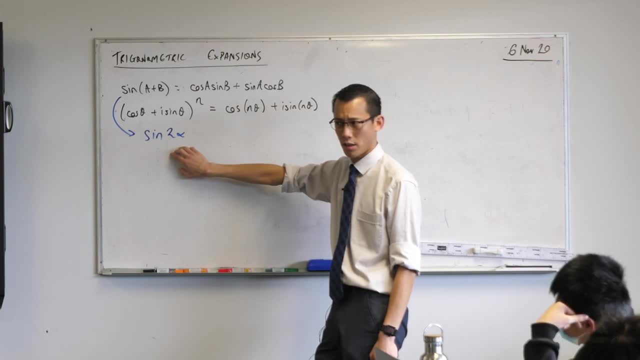 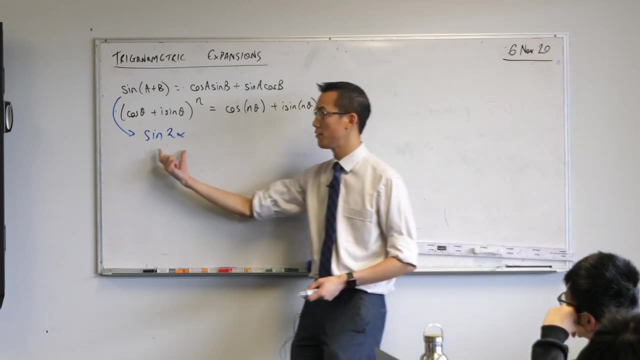 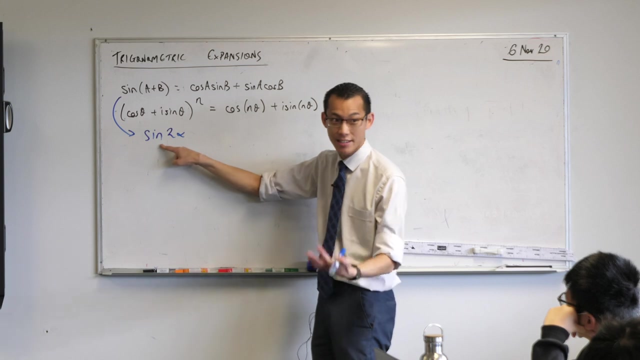 For this. What am I going to need to substitute in? Have a think, Have a look, Look at this line and where I could potentially find this guy. I'll just put it to you rhetorically, right? Do you think you're going to get this guy easily and nicely from that term, right there? 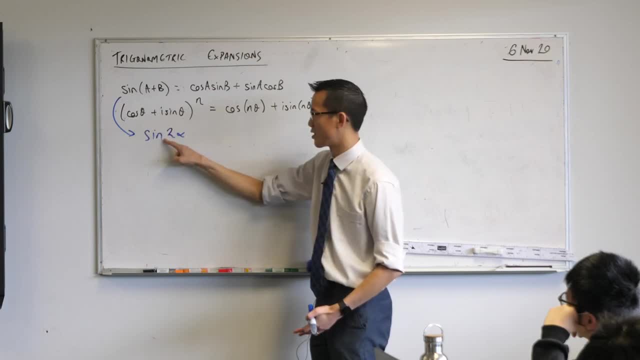 Probably not, because it's the wrong trig function, right? So it's like: okay, well, I'm going to eliminate this guy. I guess that knocks out this one as well. What about this one? Is it easy to get this? 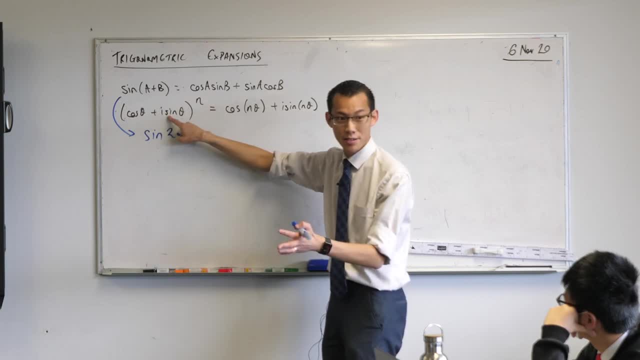 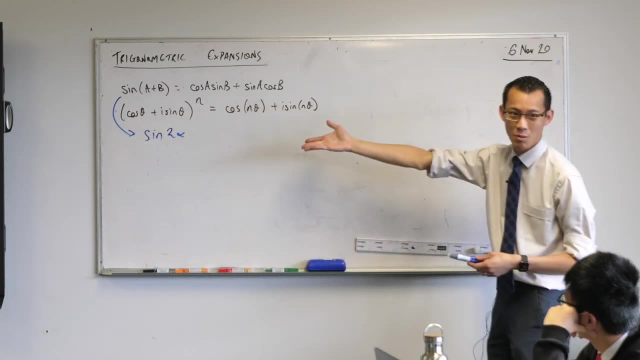 out of this. Hmm, Now some people are suggesting yes. I'm going to say yeah, we could, but it would take more work. I feel like there's an easier candidate on my equation, right. Isn't it easy to get sine 2 alpha? 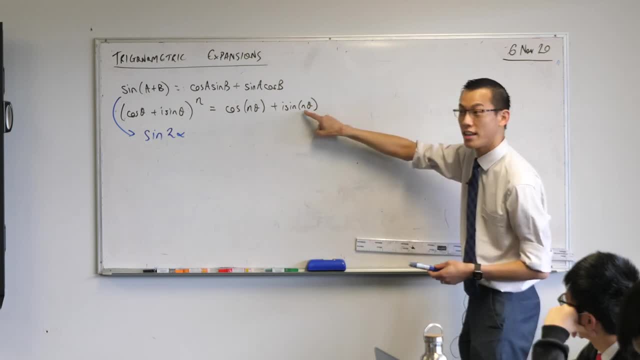 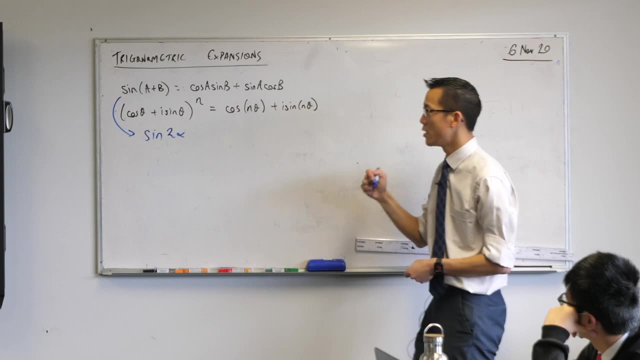 from here. Look at this. There's like an angle and it's being multiplied by something already. right, I just need to choose the appropriate thing to multiply, which is 2, right, So let's use Demarva's theorem by Demarva's theorem. 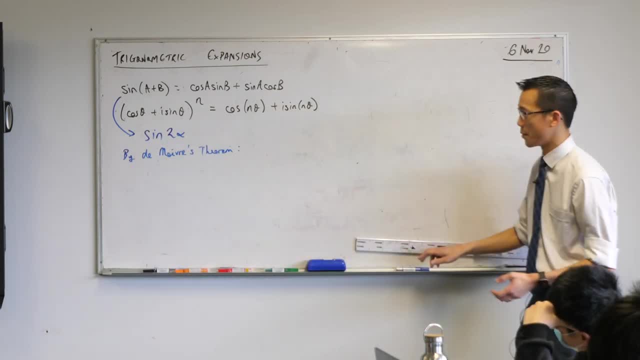 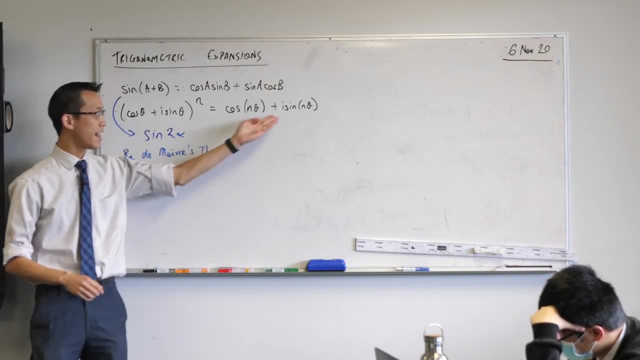 And what I want you to do is- I'm going to pause for a minute- I want you to quote it- I want you to put in the right number and the right angle to get a 2 alpha up in there. okay, It's going to mean you have to substitute a few things elsewhere in the equation as well. 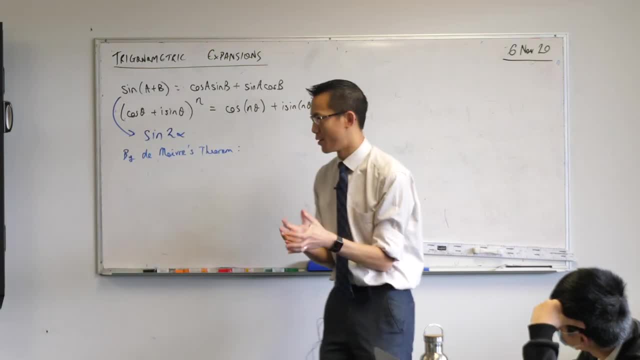 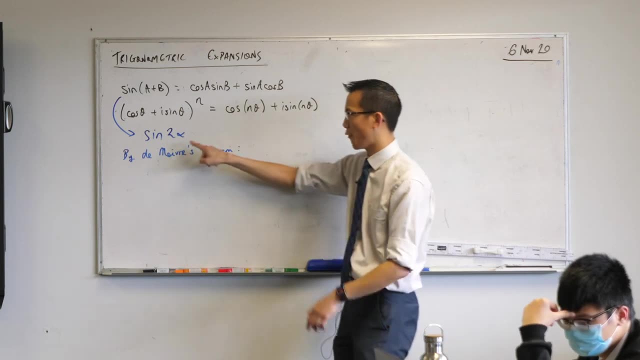 And then we're going to pull out a trick we keep on using because it's so phenomenally useful, right? You're going to get some real stuff and some imaginary stuff on this right-hand side, and because this is a sufficiently low power, right. 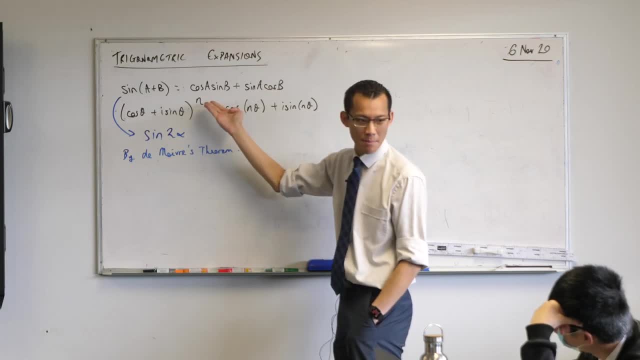 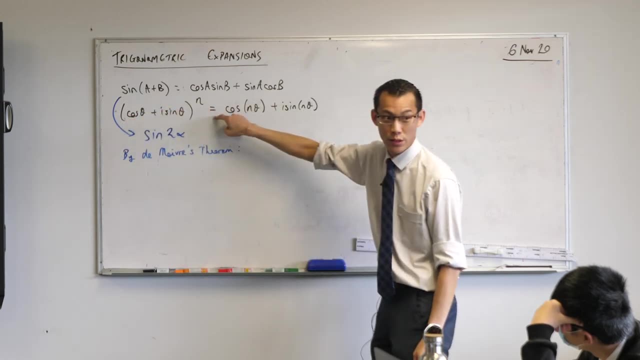 You can actually expand This guy out once you substitute that power in, And once you do that, once you expand out, you will get some real stuff and some imaginary stuff. Now, if this is true, if these things really are equal, then all the things that are. 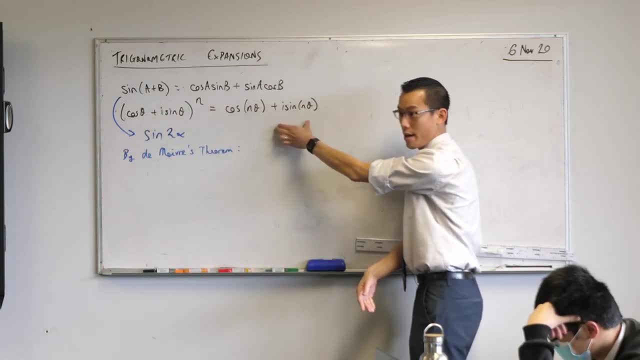 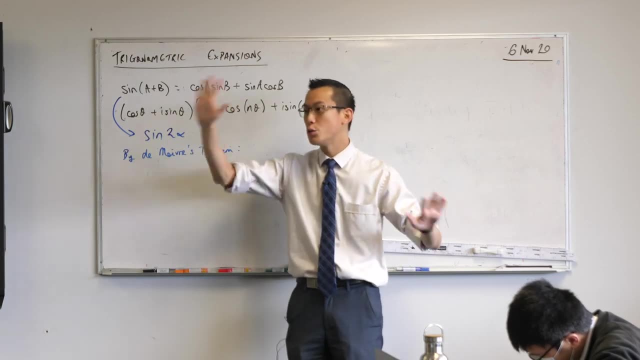 real here should be equal to all the real things that are here, And the same should be true of the imaginary things. Does that make sense? So I'd like you to go ahead, do the substitution, you expand out and then do your comparison. 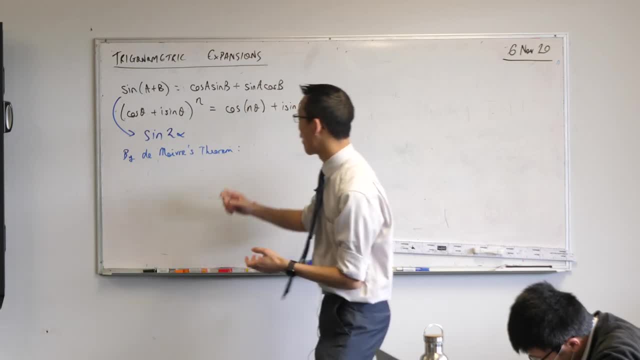 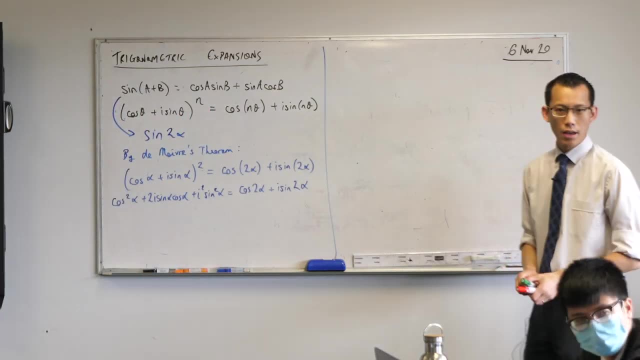 Do all the lines and see what you end up with. Remember where we're trying to go And call me over. If you've either got a problem or you think you've got a result, Off you go. So I see a bunch of you have gotten there, which is great, right. 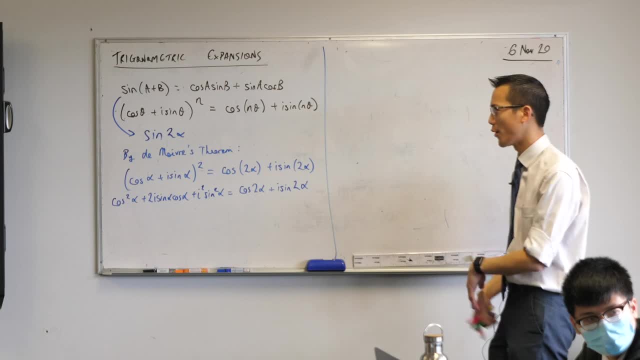 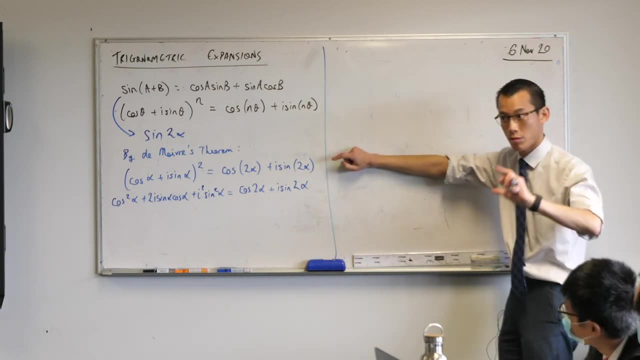 Let me just for those of you who are floundering a little bit- you're like, I'm not sure where I'm going. Let me help you out. okay, What have I done? Line one: I have quoted DeMarva's theorem. 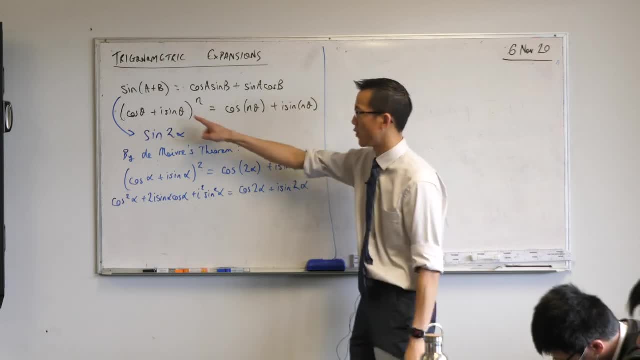 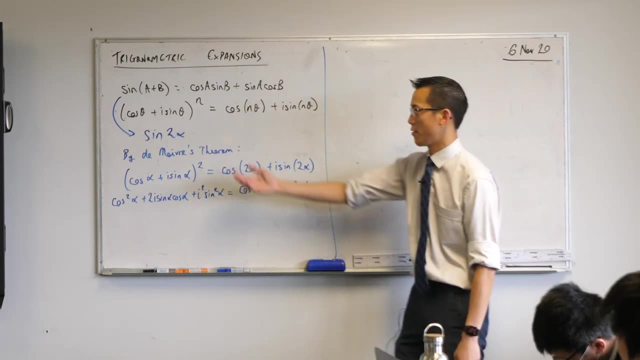 but what I've done is I've put in a particular value for theta and a particular value for n. My n is 2, and you can see here 1,, 2,, 3 times, and then instead of theta I have alpha, just to indicate like I'm looking at a specific angle here, not just some general angle. 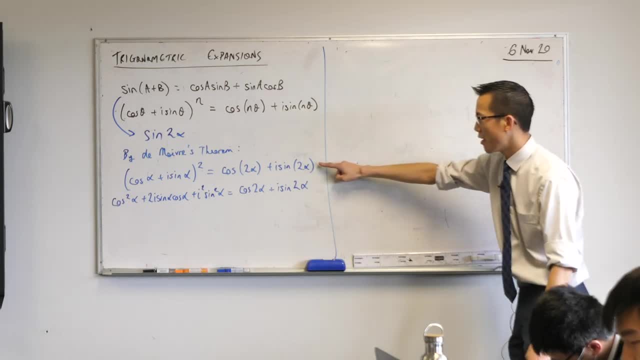 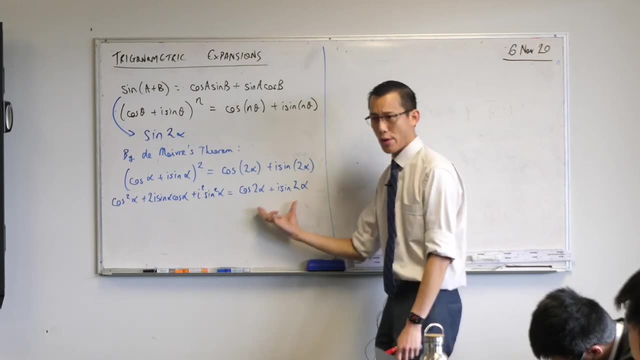 So there's my substitution straight into the formula and then from this first line to the second line. I didn't have much to do on the right-hand side, and there's a good reason for that right. The right-hand side already has the thing that I'm after This guy here, sine 2 alpha. 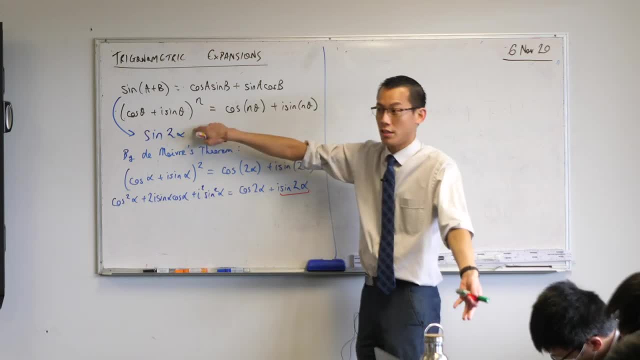 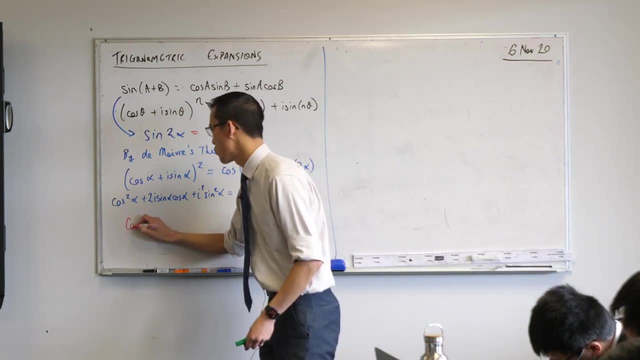 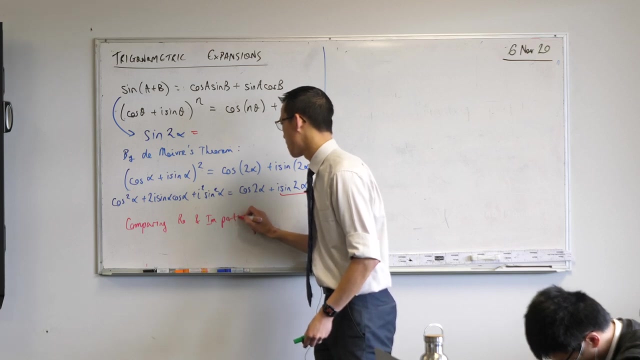 I'm just going to highlight it there. Right, This is the thing I'm actually I've been interested in from the beginning, right? I want to know what this thing is equal to. okay, Now I can actually say- and I hope you wrote this down, by the way- comparing real and imaginary parts. 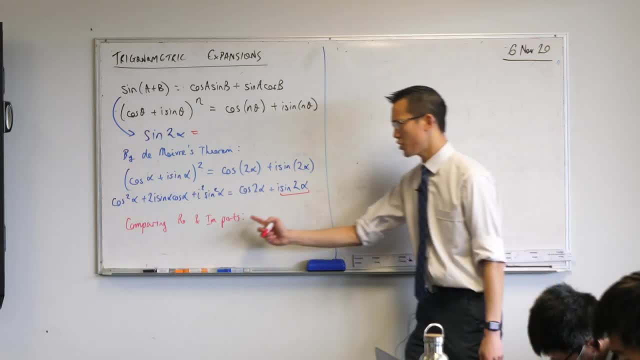 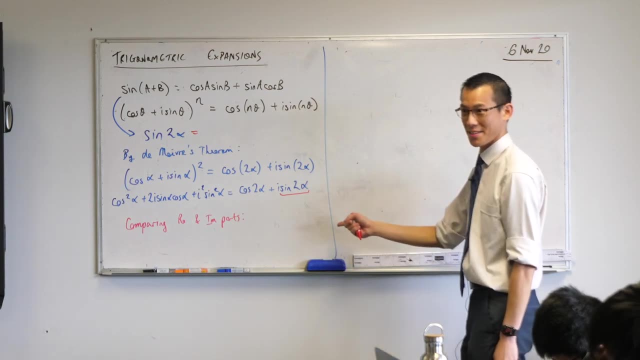 to get to this sine 2 alpha. which which of these does it represent? on the right hand side, the real and imaginary? have a look at the thing that's attached to the front of my sine 2 alpha. that's an eye right. so it's the imaginary part that. 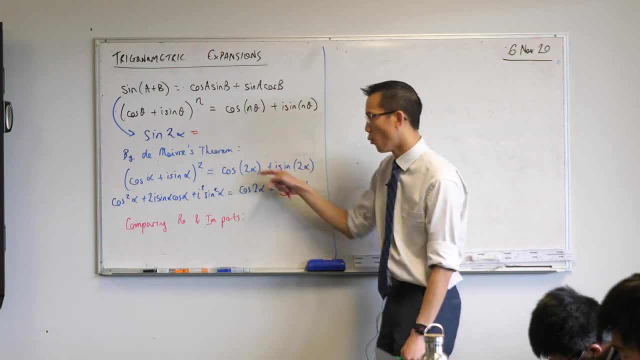 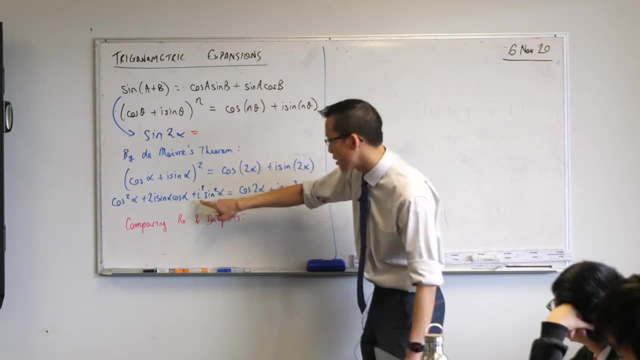 I'm particularly interested in to try and get an answer to this. so what is the imaginary part here? well, I actually already have it on the left hand side, even if I haven't finished simplifying. you can see that I squared there because we're squaring I. it's going to take me back into the real world, so therefore, 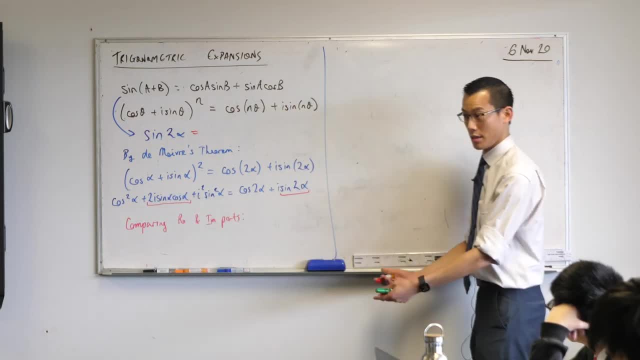 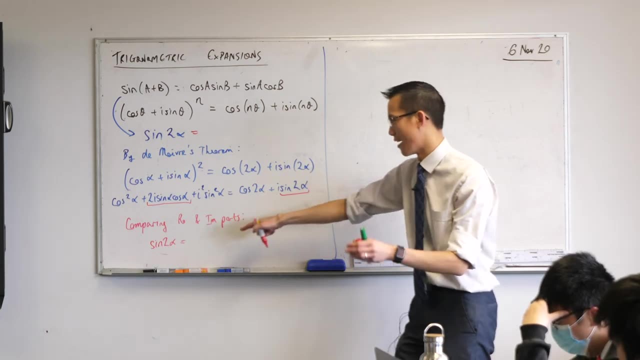 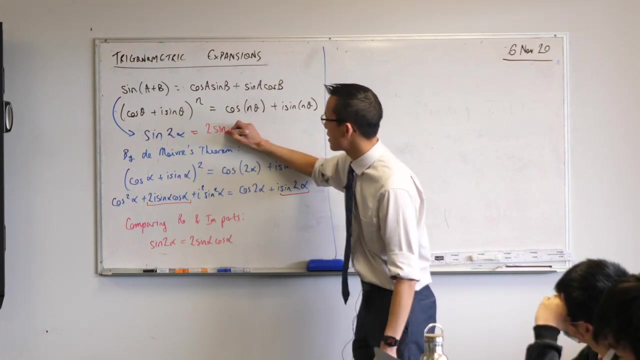 this bit. here is the one I'm interested in. do you see that? so I can just say sine 2 alpha. remember the imaginary part actually doesn't have the I attached to it when I write that equals 2 sine alpha, cos alpha. now why does that make sense? 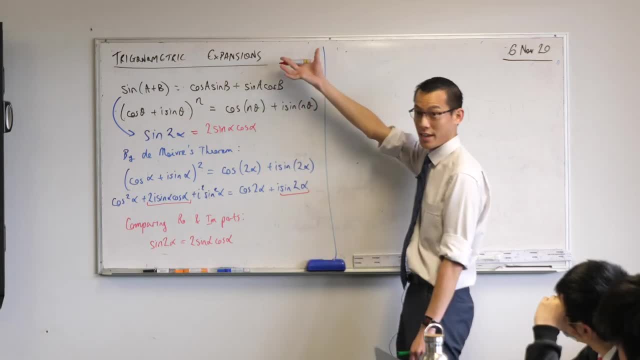 of what we're going to do here is we're going to take this sine 2 alpha and we're going to go straight over to the real world, which gives us a perspective of what we started with above. well, if we just did the substitution from here which we 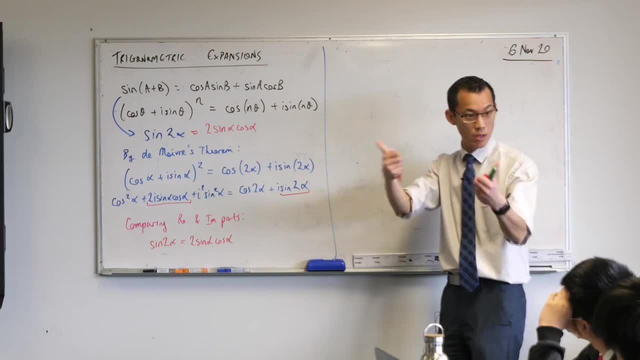 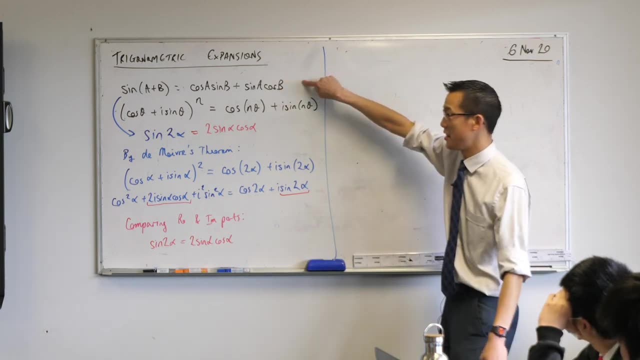 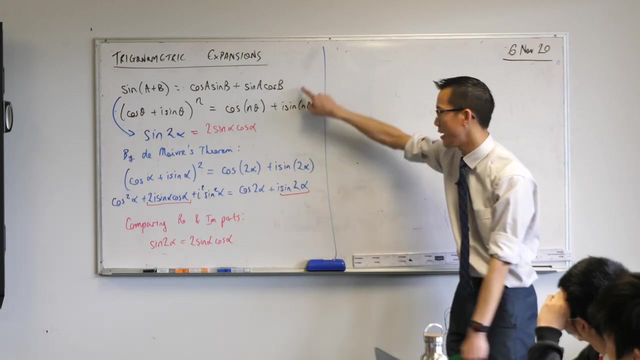 didn't know why. it was true, you get cos alpha, sine alpha, plus sine alpha, cos alpha- the same thing. so you got two of them right. so you're like: sweet, it works okay. now, what's great about this is two things. number one: ninety percent of you said this I'm fine with, and I have no idea why it works right. 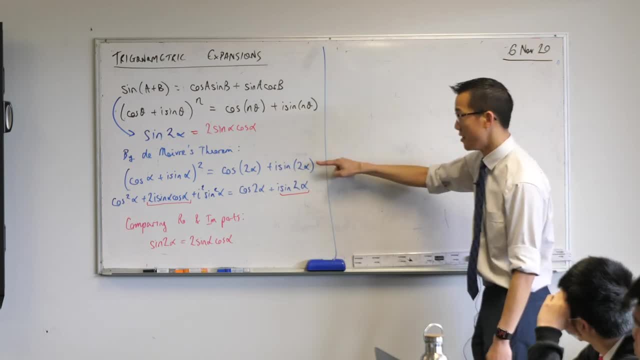 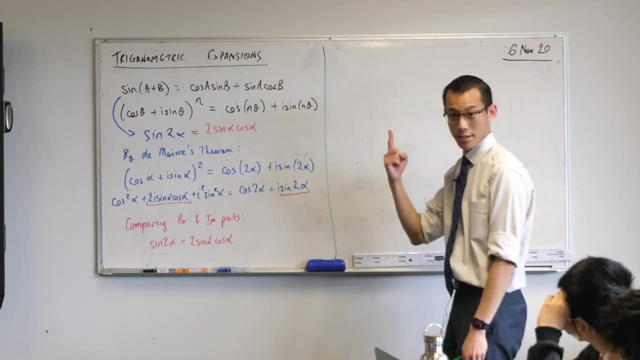 but I hope you're able to trace back in your mind by going back through this thing- right, This is true because I got it from here, which I got from exponential form and so on- You have a strong foundation to live on. That's the first thing which I want to point out. 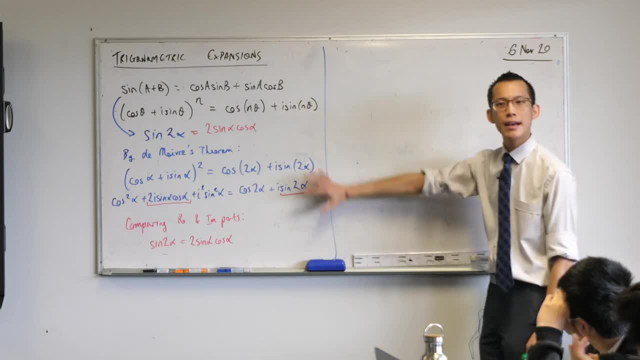 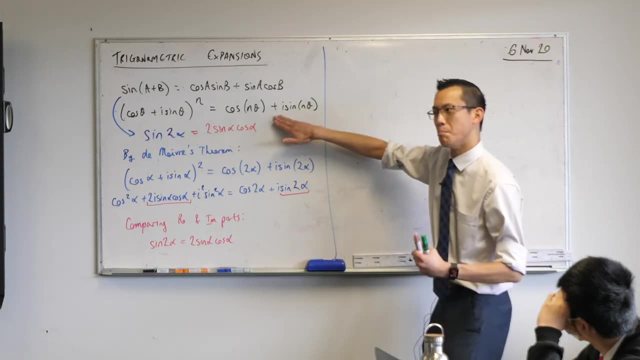 Actually, I'm going to point out three things. Second thing I want to point out is you never had to do any diagram or geometry or geometric reasoning here, because all the geometric reasoning is baked into the results that we started with. right, All of these, and you go all the way back. 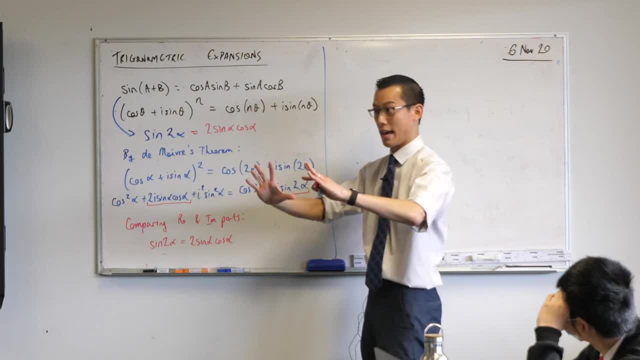 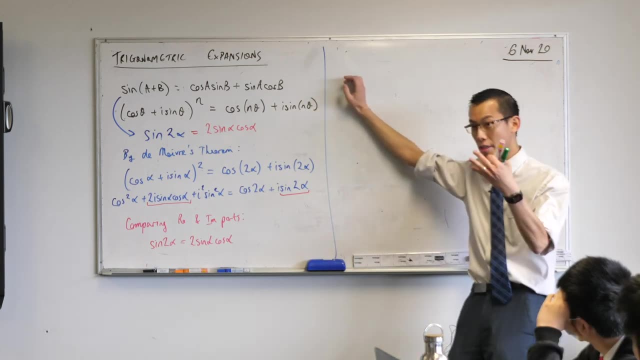 We've been doing trigonometry and drawing diagrams on the complex plane all the way through this topic. So it's kind of like you get that logic for free just by quoting a line like this, right? And then the third last thing is you get a result as a bonus, right? 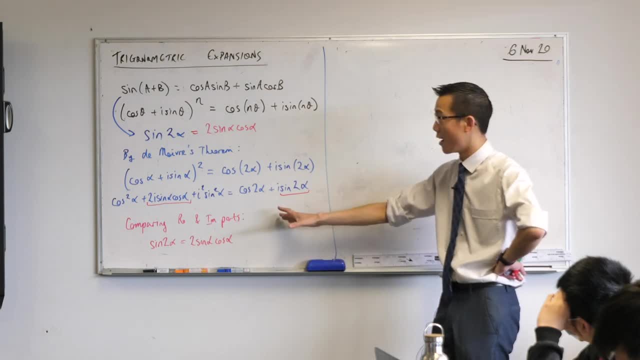 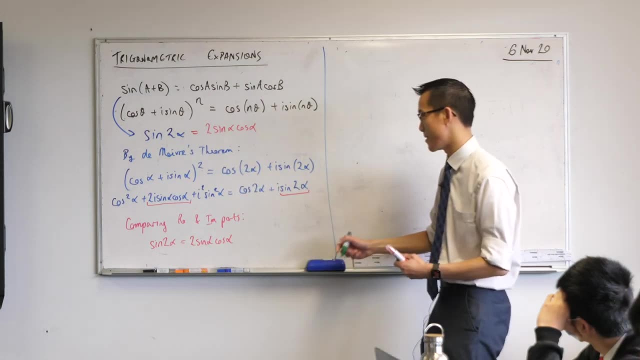 Because this is the real and the imaginary parts together. I haven't touched the real part, right, But I set out to try and find out what sine 2 alpha was. but now we get cos 2 alpha for free. It's right here, right.